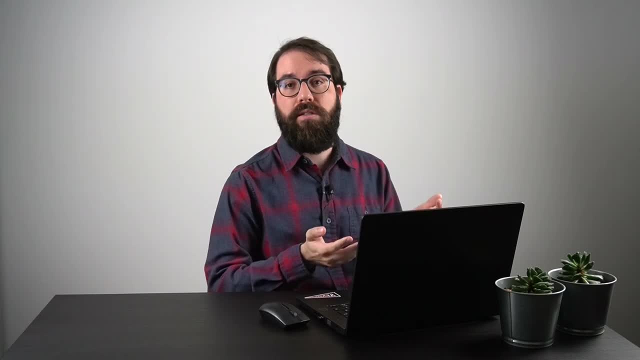 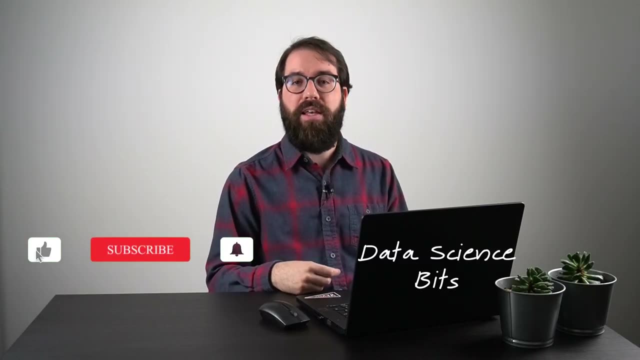 curve, what's useful for and what are the limitations, And also, in the end, I will provide some alternatives to the rock curve. My name is Felipe. this is the Data Science Bits channel. Please subscribe and click on the bell button to receive notifications with. 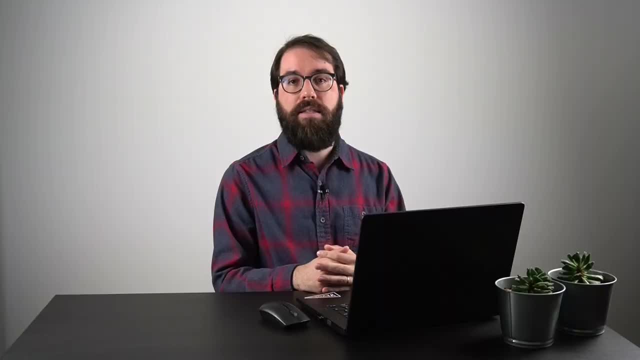 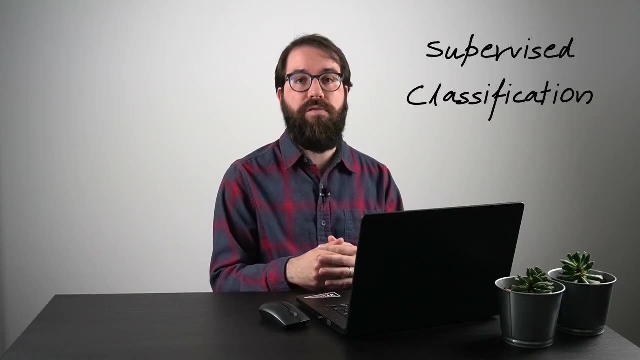 every video that I post. And let's begin. As I already said in the introduction of the video, the rock curve is used for classification models, and especially must-be-supervised classification models. So you have classes A and B, or let's say negative class and the 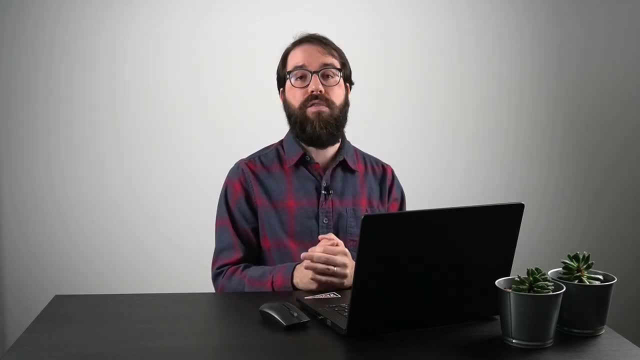 positive class- this is the usual notation- and you have a validation set that you have been holding out from the computer And in this validation set you have the predictions of your model and you also have the actuals. So throughout this video you can imagine. 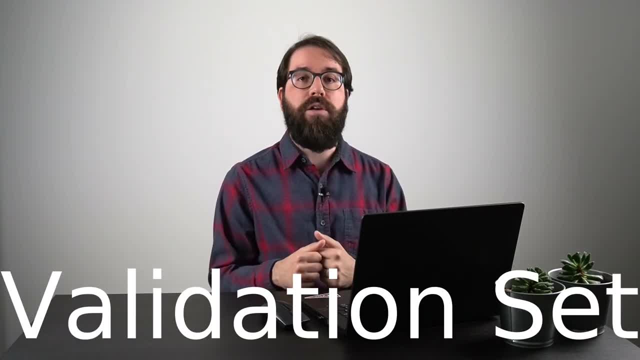 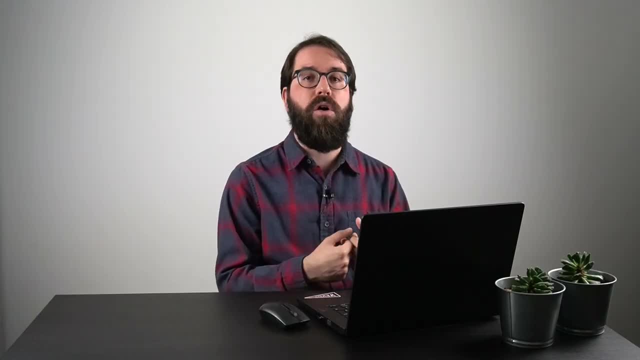 that we are going to talk about the rock curve and we are going to talk about the validation set, where you are checking the performance of your model to finally test it out either in the field or in a new test set. I have a surprise for you. I prepared 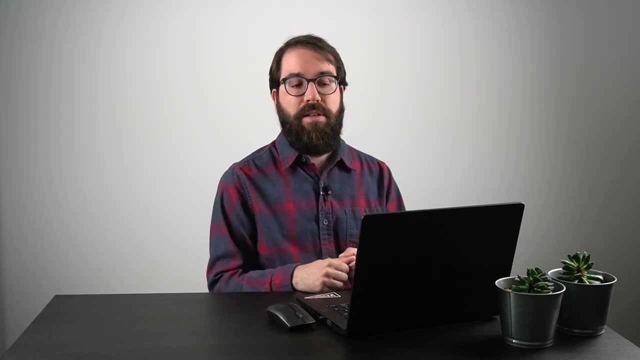 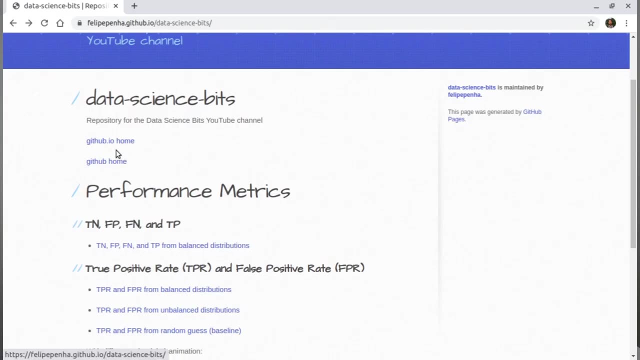 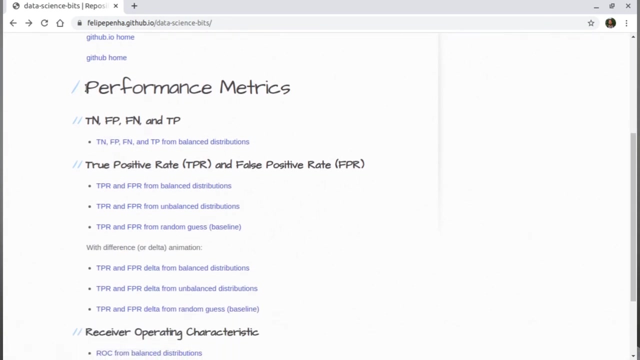 a website with supporting materials to this channel. So let's take a look. So it's githubio slash data science bits. You can access the repository, where you will find codes and the original HTMLs, And I prepared a section here called performance metrics that will serve for the series of 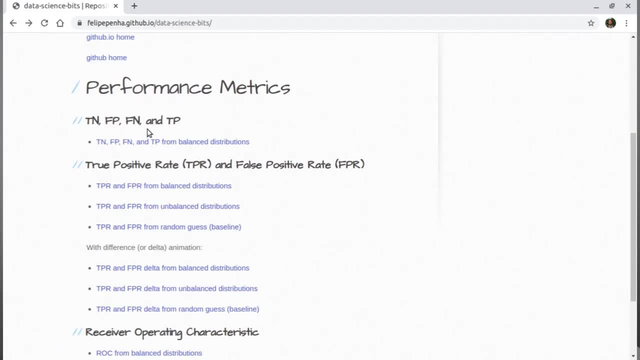 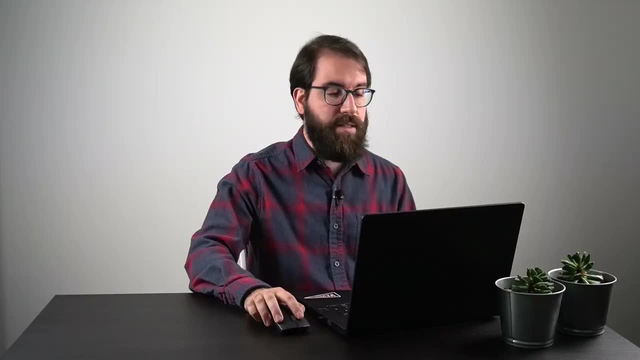 videos that I prepared on performance metrics And in special. now we will talk about true negatives, false positives, false negatives and true positives. So let's dig into that. You have your predictions and your actuals So you can plot a distribution for the actuals. 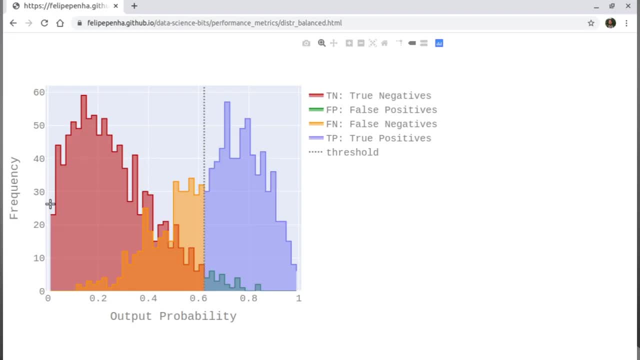 of the negative class, That's the red curve plus this tail here. Okay, so this curve here And you can also plot the distribution of the positive class, actuals, And this is all this curve here, This is the tail and this blue curve, These two distributions. 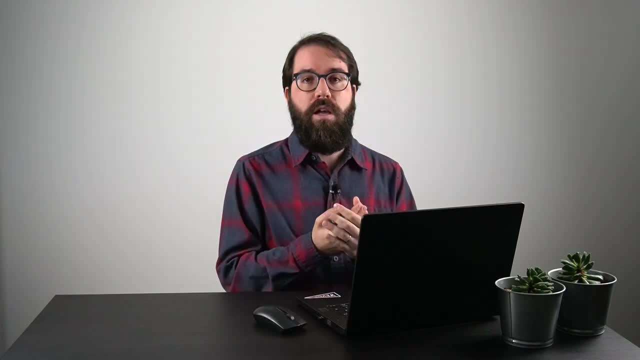 they will cross because the model is not perfect. If the model was perfect, the two distributions would be far apart from each other, accumulated in zero and one. because in the x-axis you have the output probability, You must choose a threshold where it will split the model between negative class and 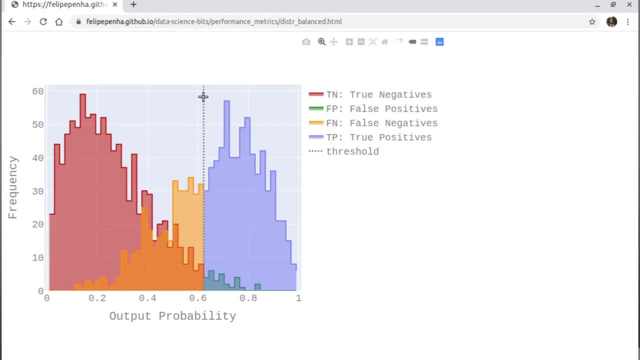 positive class. This is the dashed line here. Everything below is negative. Everything above the dashed line is predicted as positive. So you see that this red curve: here everything is negative and it's being predicted as negative. So these are the true negatives, the TN here. 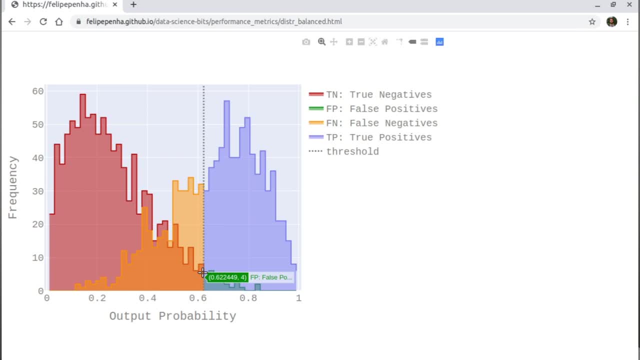 Then you can keep going forward in this curve where the actual negatives are actually being predicted as positives because they are above the threshold. This is the green curve. here. The green curve are false positives because we know they are negatives, but we are predicting. 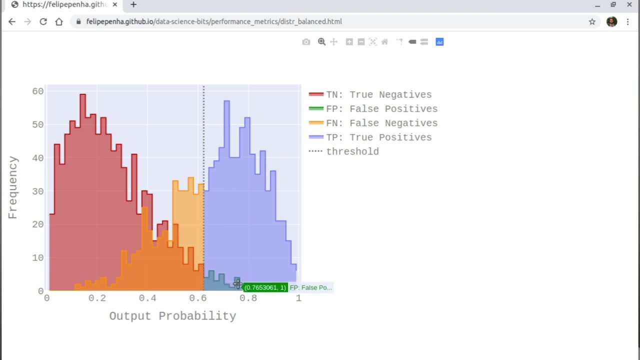 them as positives, So these are the false positives. The same for this curve: These are actual positives and they are being predicted as positives, So they are the true positives. When you go below the dashed line on the orange curve, here these are positives and we are predicting them as negatives, So they 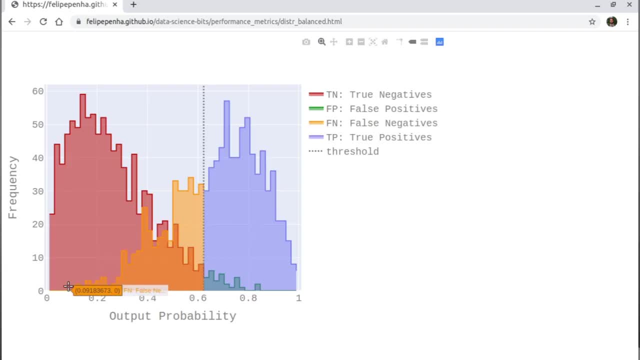 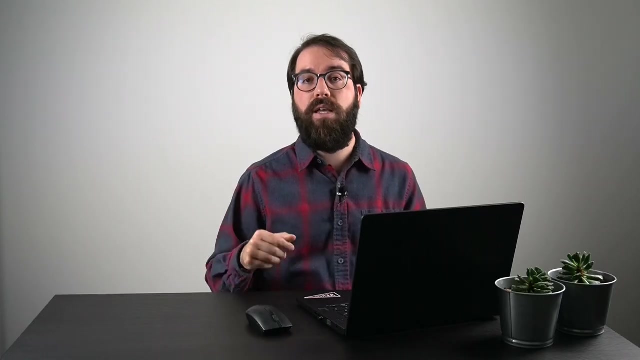 are false negatives. Okay, and you move the threshold and these proportions of true negatives and false negatives, true positives and false positives, they will change according to the position of the dashed line. With these four values, we can define various different performance metrics. We will focus. 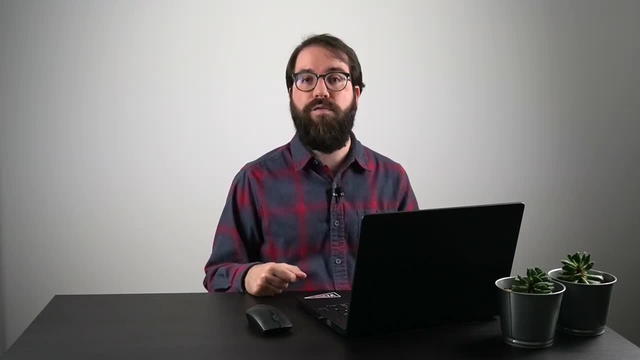 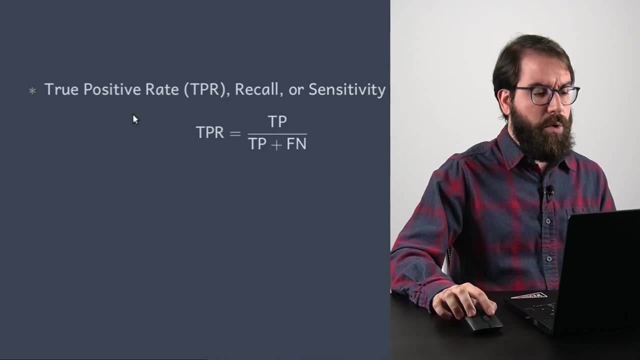 here in this video, in two. that are the true positive rate and the false positive rate that define the rock curve. So let's take a look into these definitions. The true positive rate is also known as recall or sensitivity. It's usually represented as 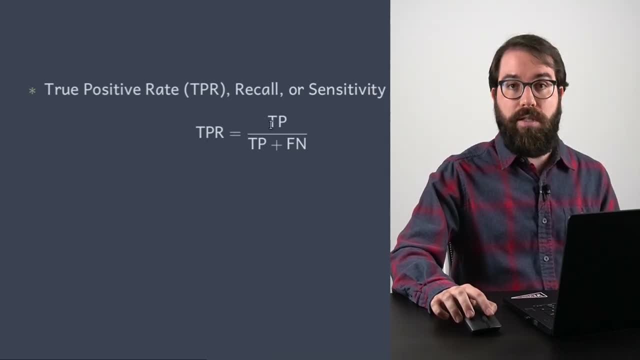 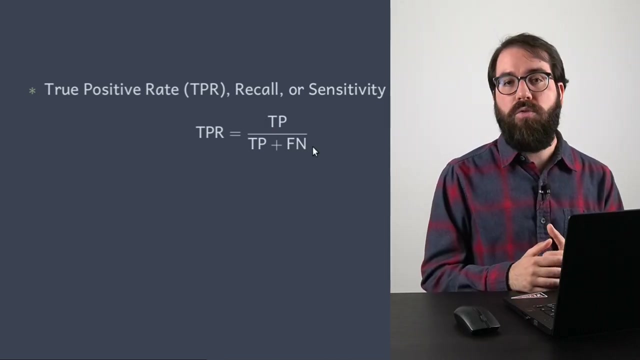 TPR. The TPR is the true positives over the true positives, plus positives. So this is basically the amount of true positives over what should be predicted as the true positive. So that's why it's called recall. It's how the model is recalling the truth from what? 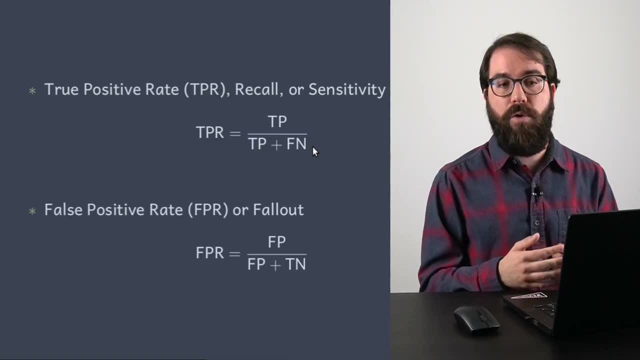 it should be. The other metric is the false positive rate, FPR, also known as fallout. So it's basically what's falling out of the true negatives. We have already seen that if we choose different positions in the threshold, we get different proportions of these quantities. So let's see what happens. 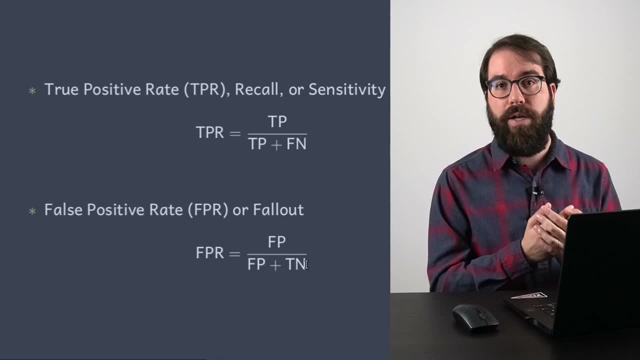 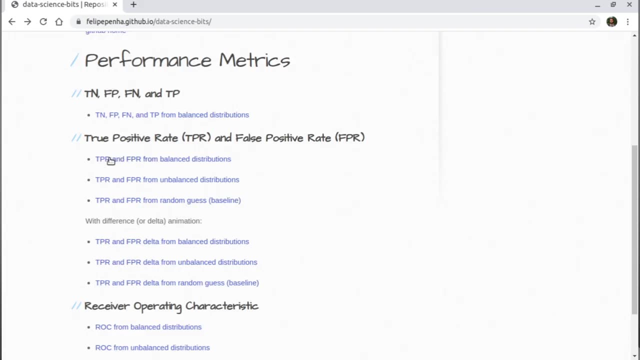 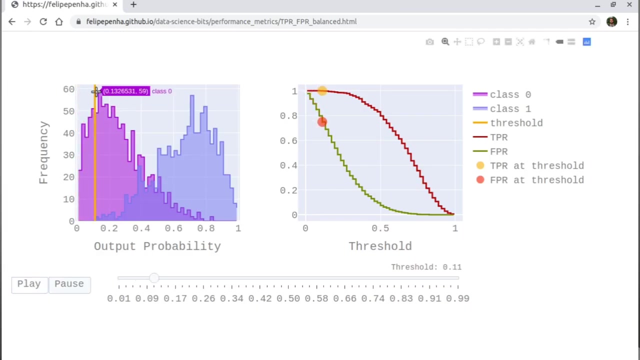 when we plot the true positive rate and the false positive rate against the threshold choice. Going back to the website, we can see here TPR and FPR for balanced distributions. I prepared here an animation. The threshold, that's the vertical orange line, keeps changing. 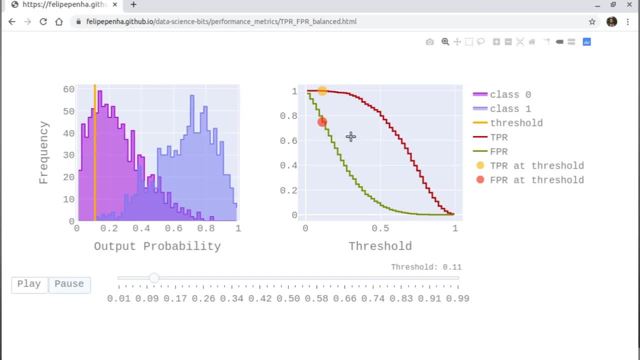 keeps going forward, And you can see here on the right, the TPR. the true positives are in red and the false positives are in green. It's easy to understand why they are stepwise functions: because the histograms have a bin size that's, in this case, is constant, So the threshold moves and it only makes a difference when. 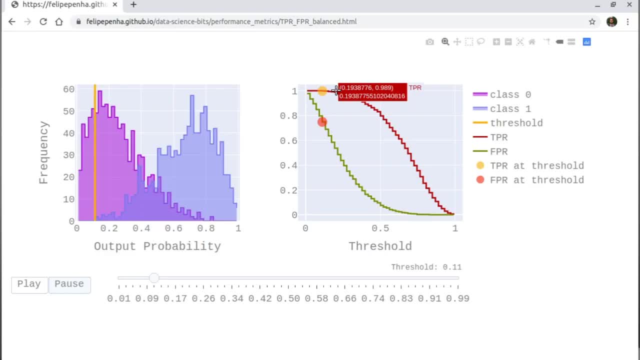 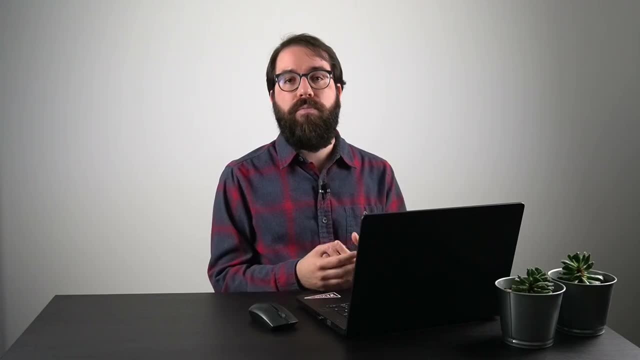 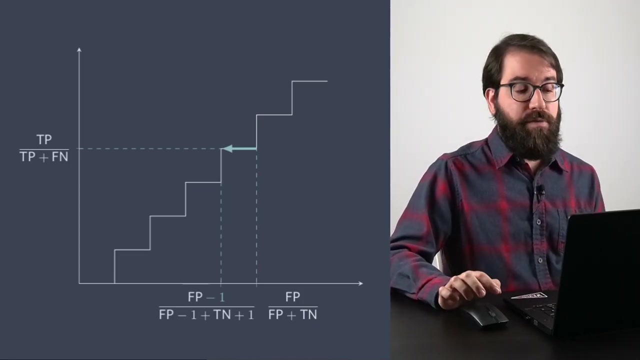 it goes forward the same distance as the binning size. I already told you that the rock curve is a stepwise function And we need to understand now how to build the curve and how it naturally becomes a stepwise So going to the rock curve. that's the true positive rate against the false positive rate in. 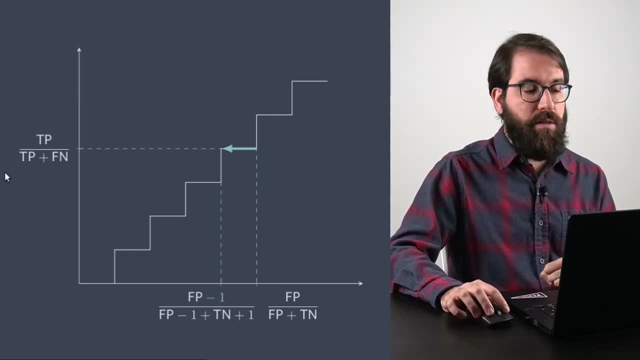 the horizontal. okay, So I already put the formulas here so we can explicitly see what's happening. You see that when you move the threshold, you are actually going in the rock curve from right to left, And there are instances where you can keep the true positives constant and also the false negatives constant, And 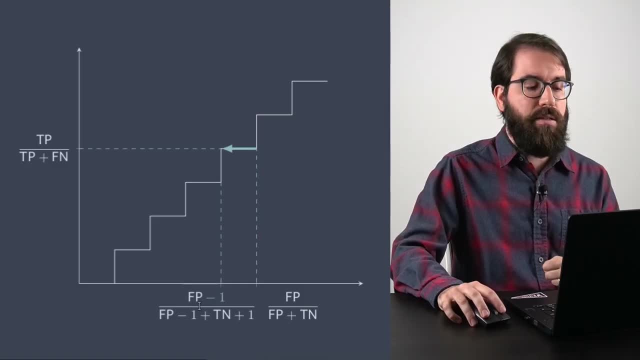 what happens is that the numerator of the false positive rate is decreased by one, while in the denominator things are kept constant because you subtract one but you have to add one. Remember, the threshold moves changing these proportions. The thing is that the denominator is always kept constant when 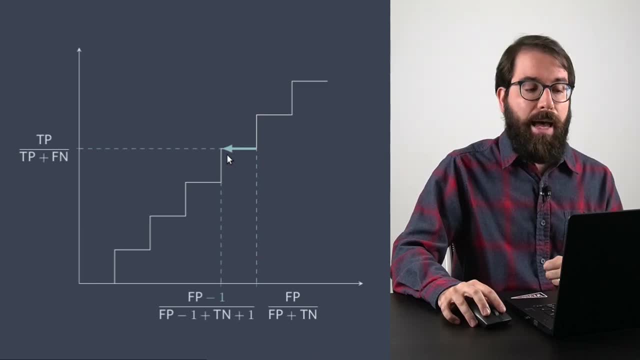 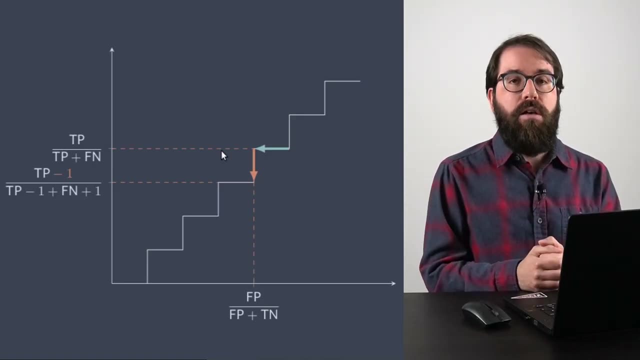 you do this. So you get a perfect horizontal line here. that is always constant. So you get a perfect horizontal line here. that is the blue arrow. And there is another situation where you can do the opposite: You keep constant the false positives and the true negatives that are here. but 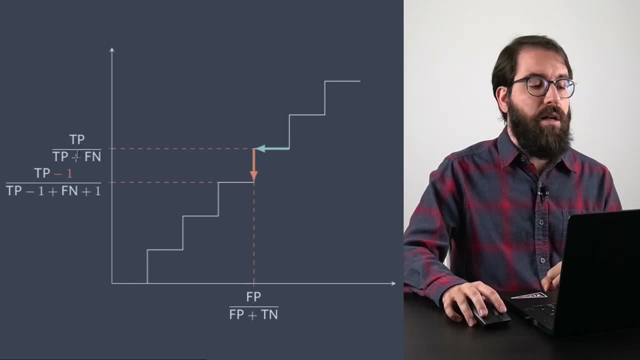 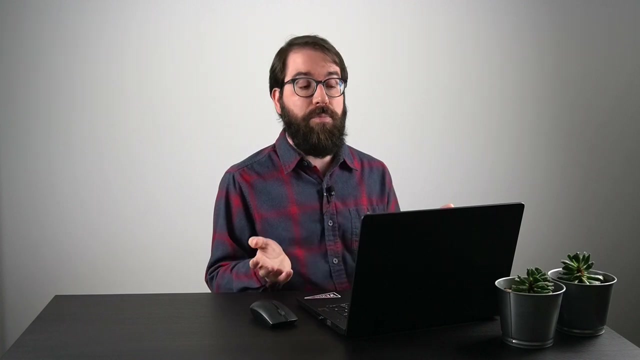 you are changing similarly to the other situation: The true positives you are subtracting one. The denominator is kept constant, because when you lose one true positive, you gain one false negative. Let's see this in action with the animations that are prepared in advance. 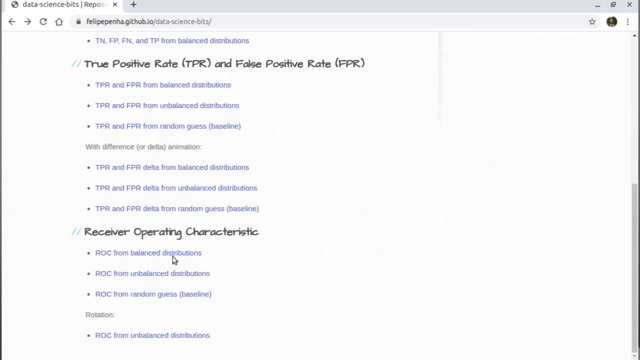 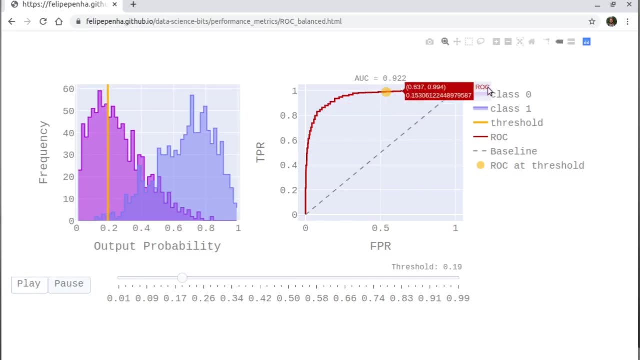 Let's see this in action with the animations that are prepared in advance. So the receiver operating characteristic here for balanced distributions. first, That's the simplest case. The threshold keeps moving. You see that the curve, the rock curve, goes from right to left. Maybe you notice a value here. That's the AUC. 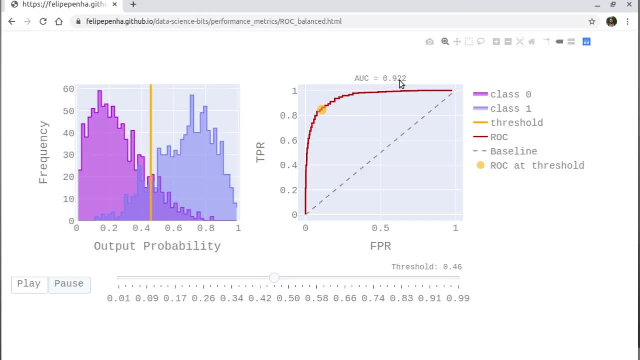 That's the area under the curve. The area under the curve is between zero and one. Why? Because TPR is between zero and one, FPR is between zero and one, So the most area that you can get is one. Okay, and then there's the diagonal line, The 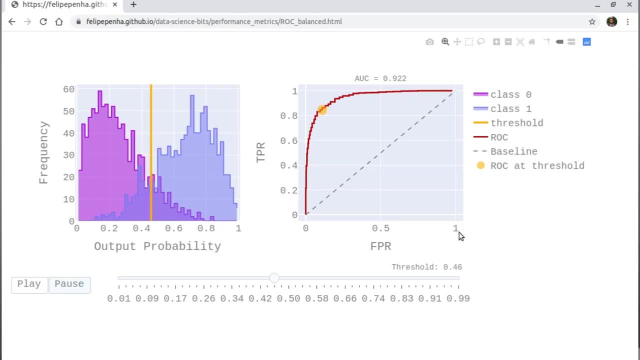 diagonal line establishes the half of this maximum area. That's 0.5.. And we are always comparing to the diagonal. That's the random guess that I already mentioned. So we actually compare 0.922 here to 0.5, because 0.5 is just the. 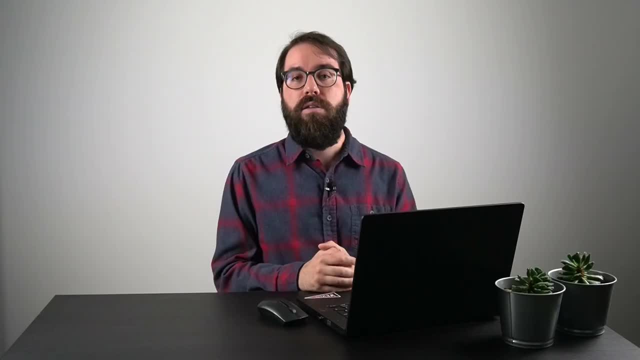 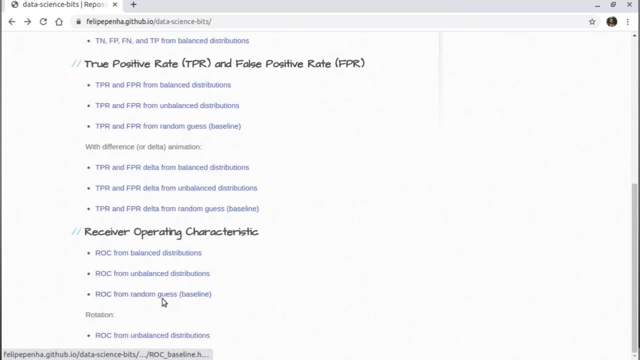 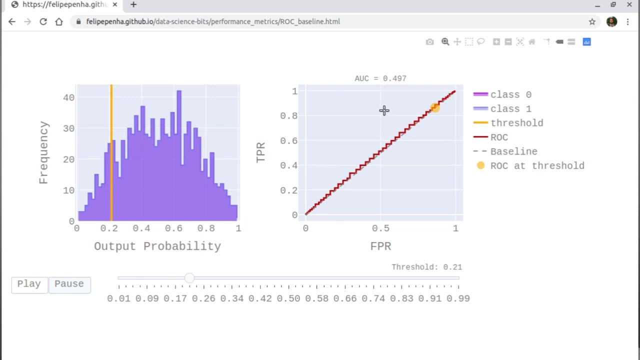 random guess. It's not a good model. So now let's understand the diagonal line. If we go back to the website, I prepared here rock from random guess a baseline. It's the same. The threshold goes from left to right, But what happens here is that I prepared 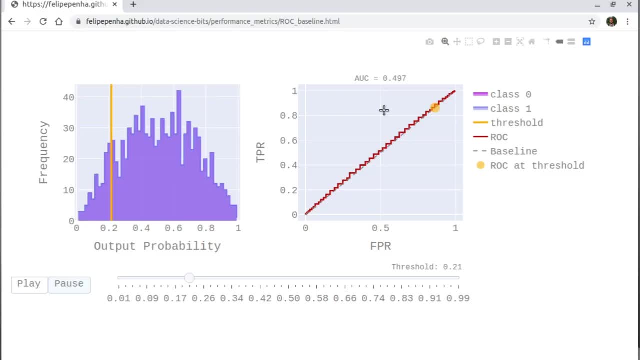 exactly distributions that are equal to each other, So they are perfectly overlapping. It doesn't matter the shape of the distribution actually. So this is analogous to flipping the coin for these two classes, And you see that if you choose the threshold, let's play again. nothing changes right. And you see that the 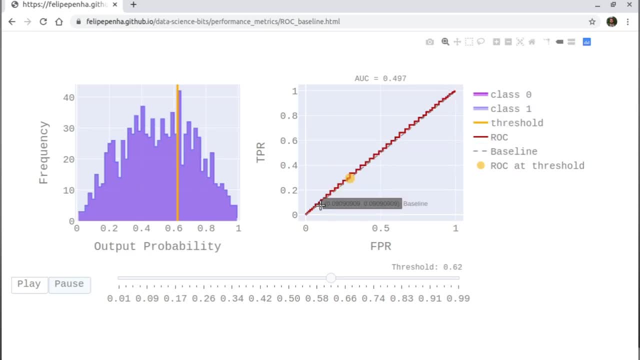 curve is always touching the dashed line in the diagonal here. If you go below the dashed line, it means that your distributions are actually switched. If you go below the dashed line, this is worse than the random guess. Let's see now what happens with the rock curve. 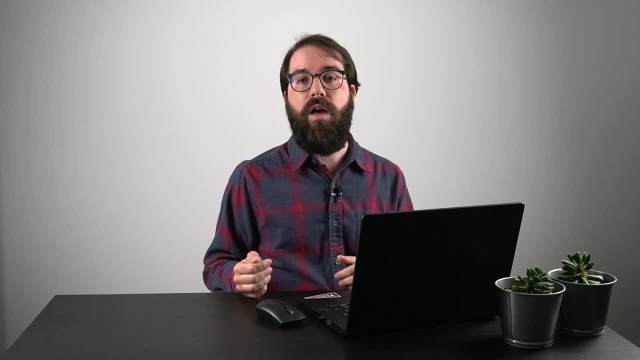 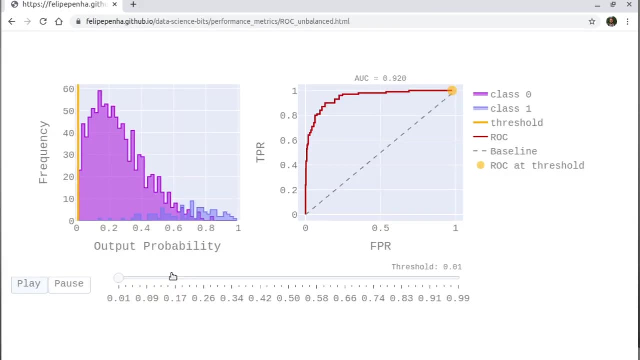 when the data is unbalanced between the two classes. So I have much more of one of the classes. So here, if you go to rock from unbalanced distributions, Let's pause for a moment. You see here that the violet histogram actually has many more counts than the blue histogram. 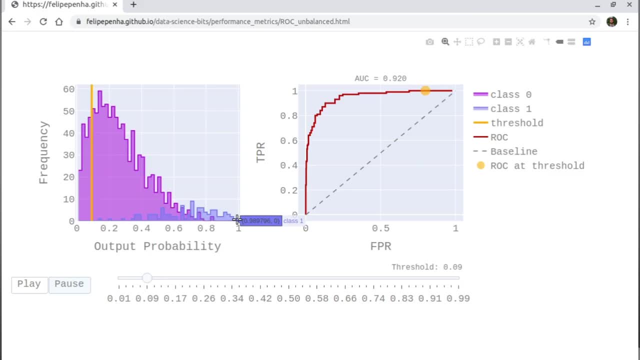 And this will make the rock curve not quite so symmetrical. So what happens is that the yellow diagram shows that when you trace a diagonal line in this direction here, your rock curve will be not so symmetrical in relation to this axis here. Okay, And one criterion. 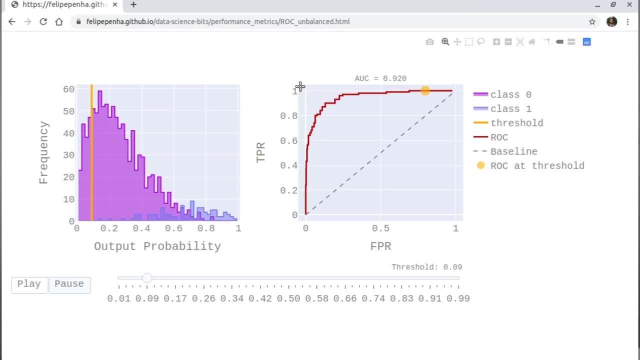 to find the threshold is the point in the rock curve that's the farthest from the diagonal line, Or in other words the closest to zero one. That's this corner. here They are equivalent. In the case of this curve, you will find this point somewhere: 0.42.. There's a very 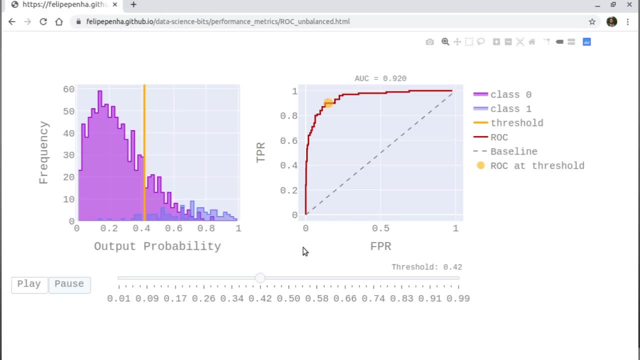 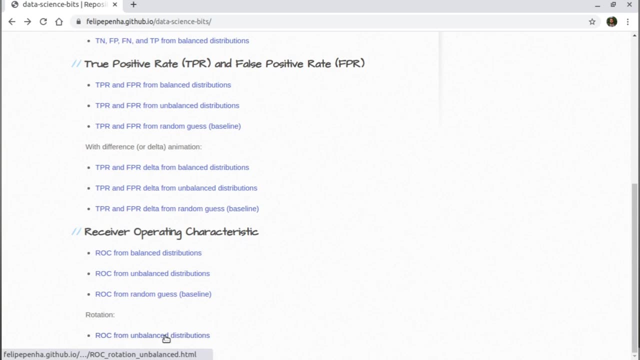 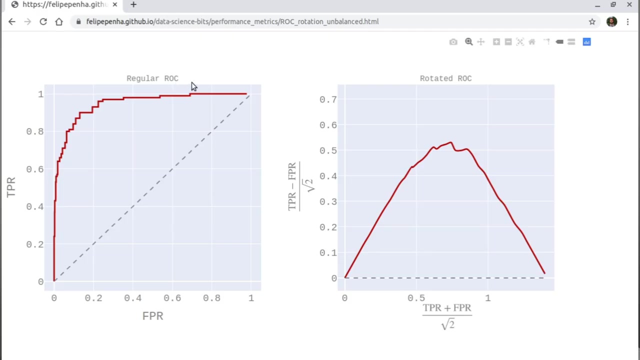 simple way to find this point, that's rotating the curve. So let's go to the website. I also prepared this visualization here. It's called rotation from unbalanced distributions. So on the left you have the regular ROC, the regular rock. That's exactly the same that. 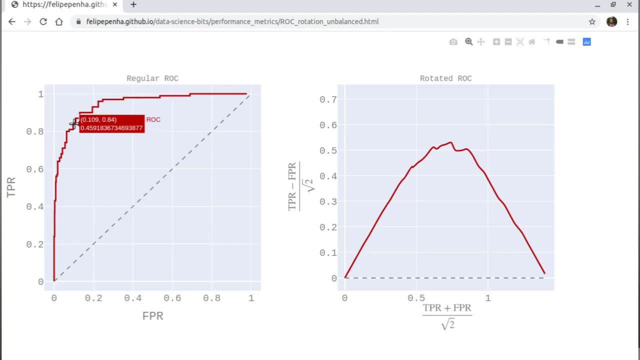 I showed before for unbalanced data, When you make a rotation in 45 degrees- because the diagonal line has 45 degrees in relation to the horizontal axis- when you make this rotation you'll see that the y-axis will become TPR minus FPR over the square root. 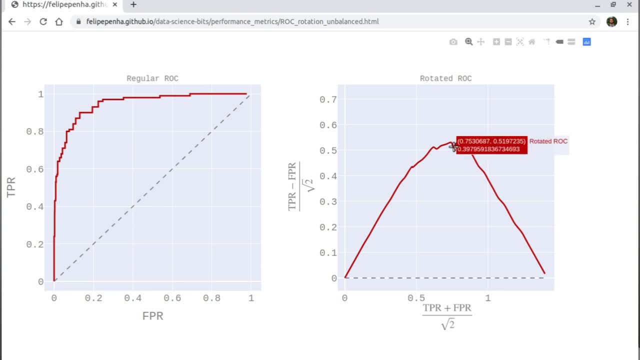 of 2.. The farthest point from the diagonal is actually the larger value of the difference between TPR and FPR. So it's somewhere here, right. As I said, it's close to 0.42.. I think it's maybe 0.418.. Now let's go back to the original curve that we showed of TPR and FPR. 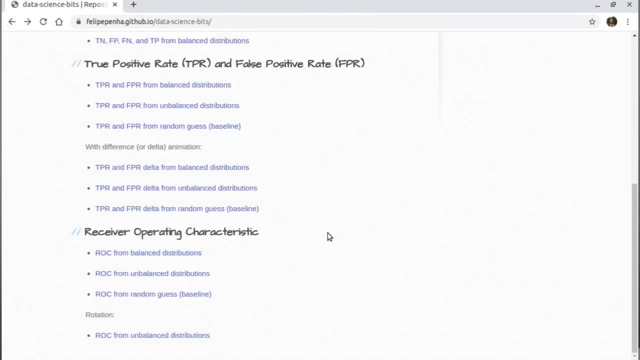 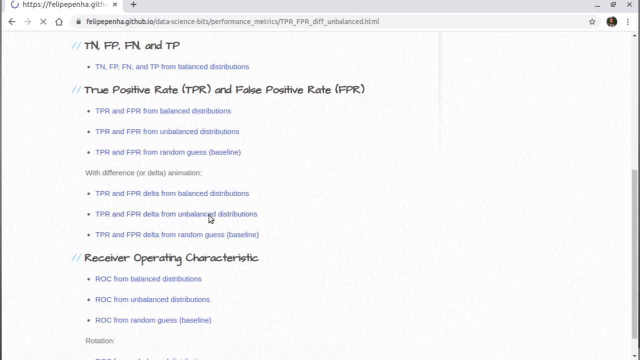 against the threshold. Let's go back to the website. So TPR and FPR from unbalanced distributions. So now I'm showing here a vertical line And I'm showing here a vertical line from the horizontal axis. And I'm showing here a vertical line from the horizontal axis And I'm showing 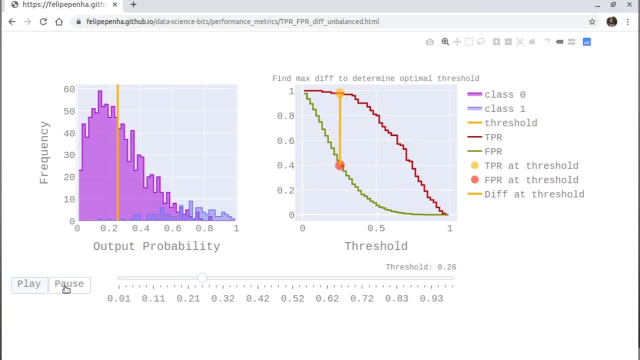 here a vertical line from the horizontal axis And I'm showing here a vertical line from the vertical axis And I'm showing here a vertical line. that's the difference, Just to visualize. Somewhere near 0.42, we will pause And this is the largest distance between. 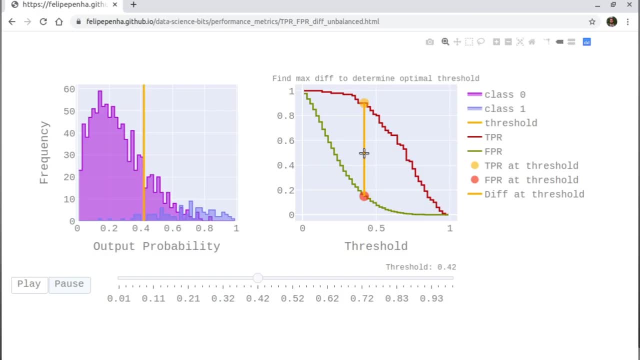 the two curves. This is completely equivalent to finding the farthest point in the rock curve to the diagonal line, And I find it easier to visualize here and to also find that point In practice. you will make an algorithm that will find this point automatically. 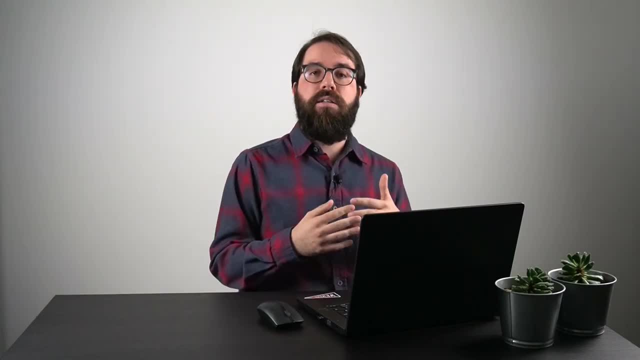 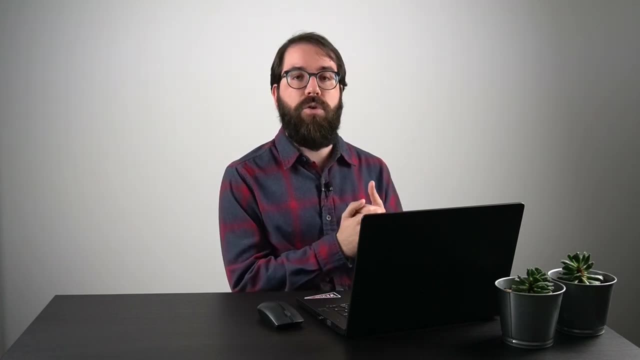 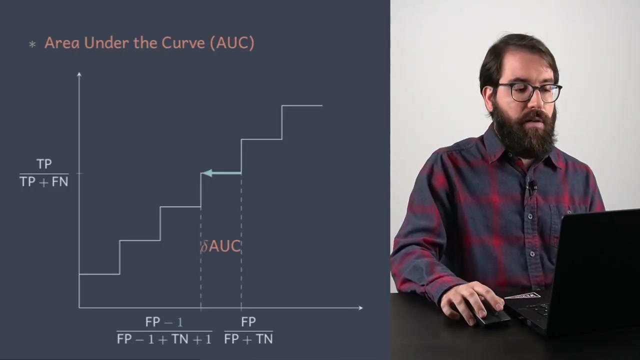 click for you. Now let's talk about the area under the curve. Let's go into more details about the area under the curve and find out what are the limitations of using the AUC. So let's take a look into the mathematics of it. So the area under the curve, or AUC, you can think of a sum of different. 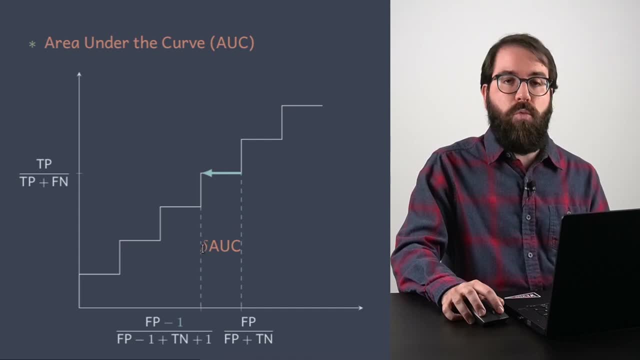 rectangles under the curve. So let's take a look at one element of area here. It's easy to understand that the vertical distance in this rectangle here is the TPR, the true positive rate, and this distance here on the horizontal is exactly the difference between FPR in this. 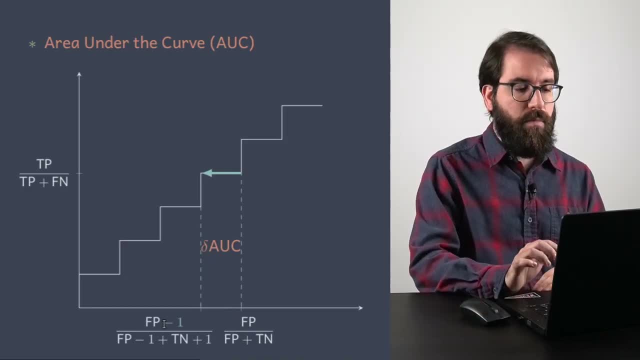 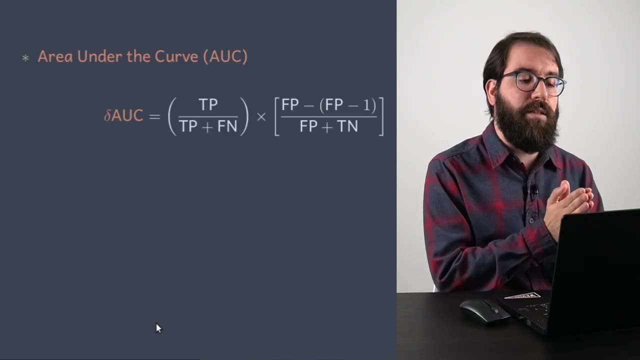 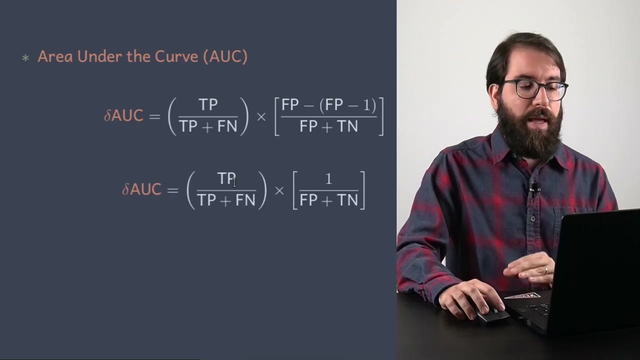 point and FPR at this other point. This translates into this formula, where I'm already making the multiplication to get the area of the rectangle. What happens is that the false positives will nullify each other. here You get this formula and I will rearrange this formula to: 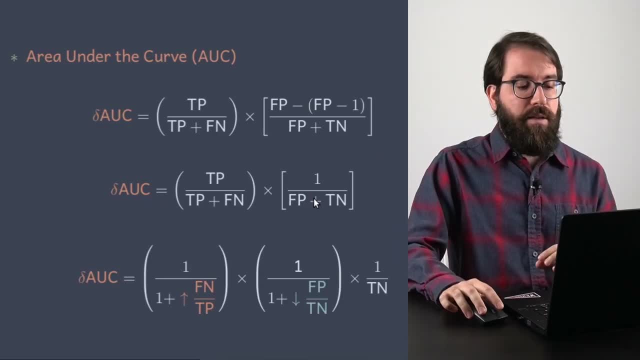 better analyze what happens If I represent the formula above in this way here. so what I did was to divide this part of the expression by TP, true positives. so I get this term here in orange and I factor out this factor here to get this other. 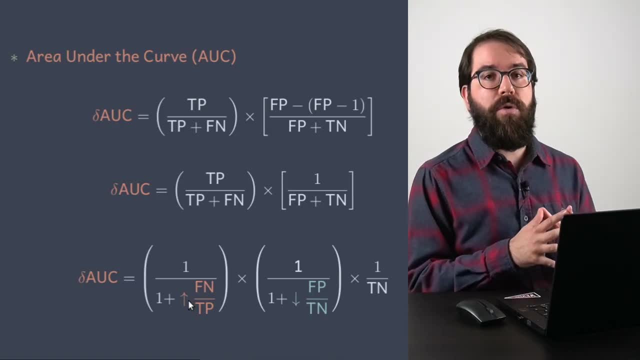 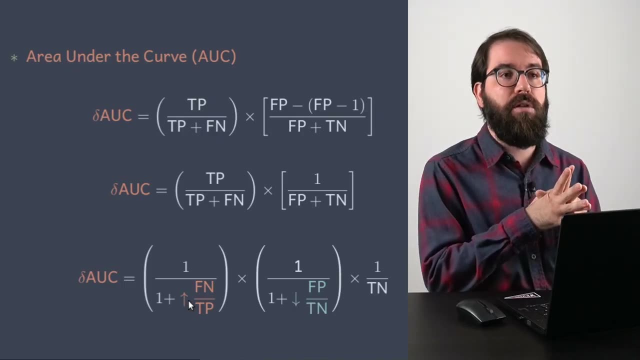 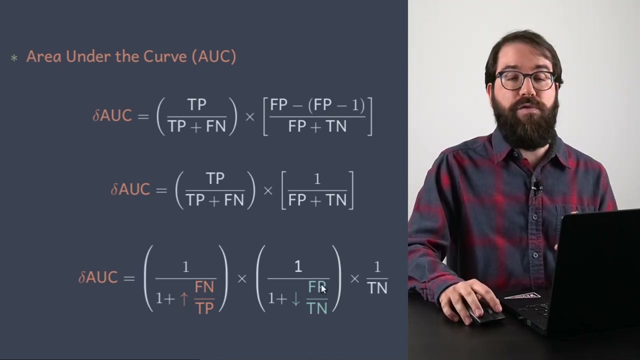 ratio. here in blue, You see that there's always a way to have different histograms. So we are not anymore changing the threshold. We are thinking about different combinations of distributions. There's always a way to increase false negatives and decrease false positives while keeping. 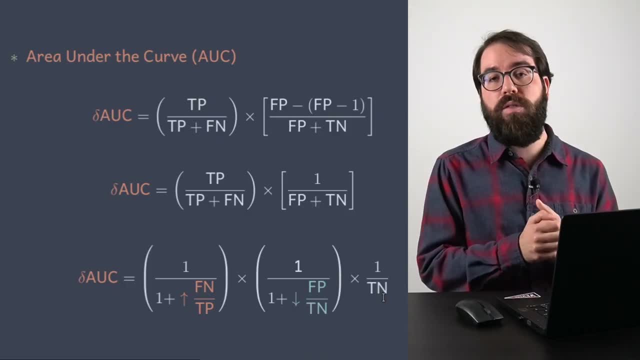 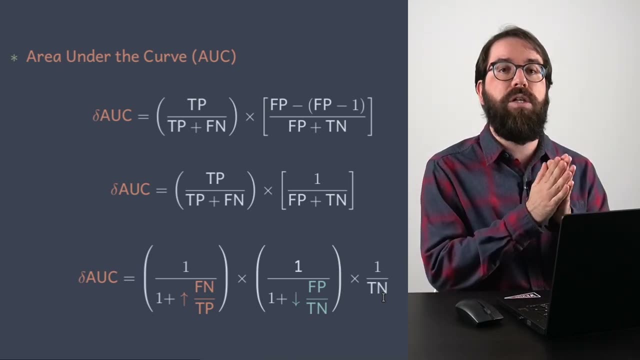 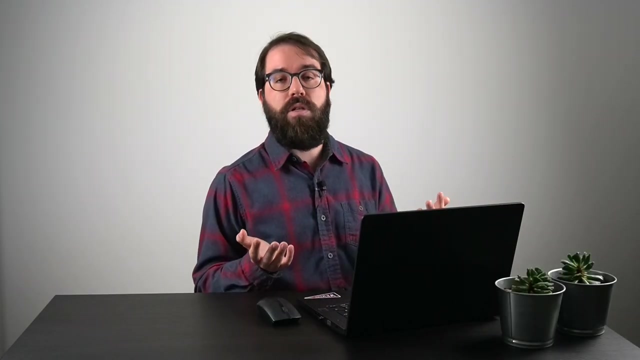 true, negatives constant, that the AUC will be kept constant. So the AUC is not telling you anything in this way. It's telling you the proportion between false negatives and false positives. This is the basic limitation of the AUC. Now let's dig into some alternatives to the rock curve and 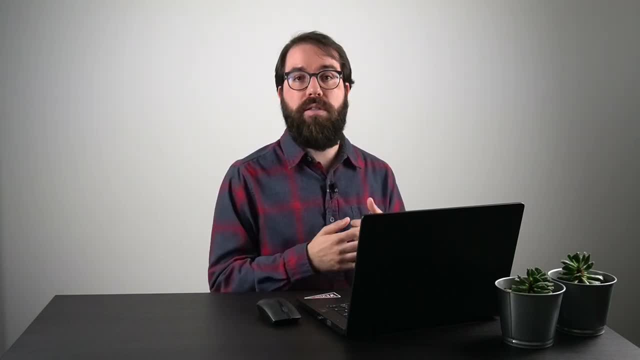 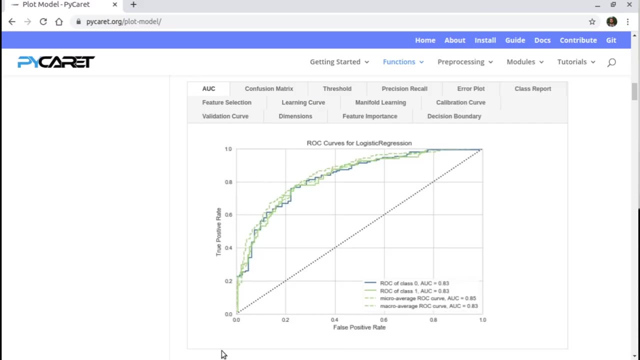 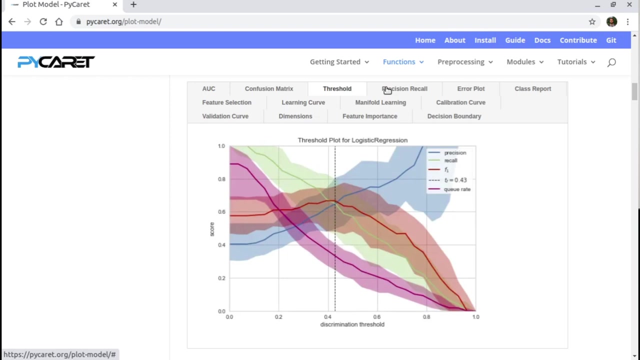 the AUC and also to find the threshold. The best source I found is the PyCaret module in Python and you can see here that it already represents automatically the rock curve with different AUCs. Let's go forward. You can find. 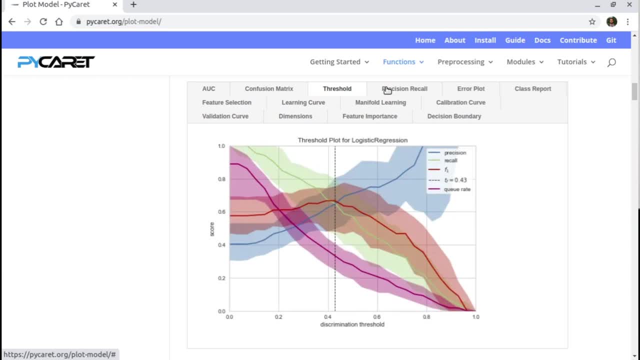 the threshold here in a very simple way. that's an alternative to the rock curve. that's plotting the precision and the recall versus the threshold on the horizontal line, and you will choose the threshold where these two curves are close to each other or where they cross. Now talking about 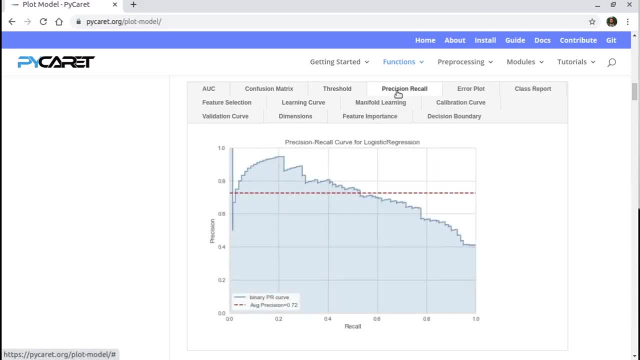 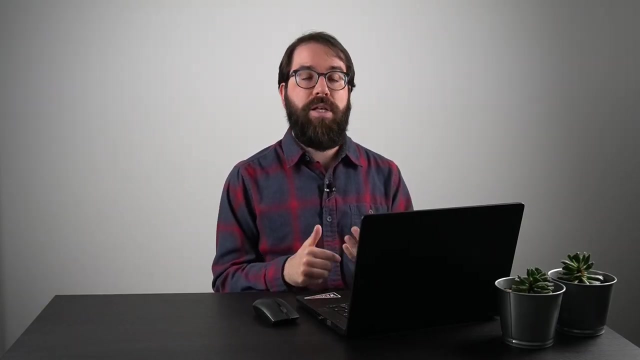 area under the curve. the precision versus recall is a better representation to get more information about the proportions between false negatives and false positives. So that's it. I think it's a lot of material for one video. I will address different performance metrics, different alternatives in future videos. 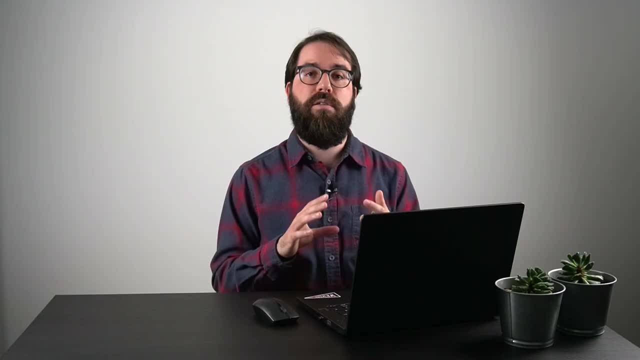 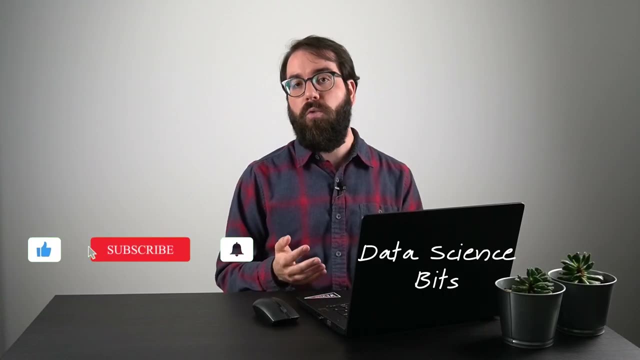 I hope to make a series. Usually I put the videos that are related to each other in playlists, so keep an eye on the playlists in the channel. Please subscribe to the channel, click on the bell button to receive notifications with every video, and also follow me on LinkedIn.